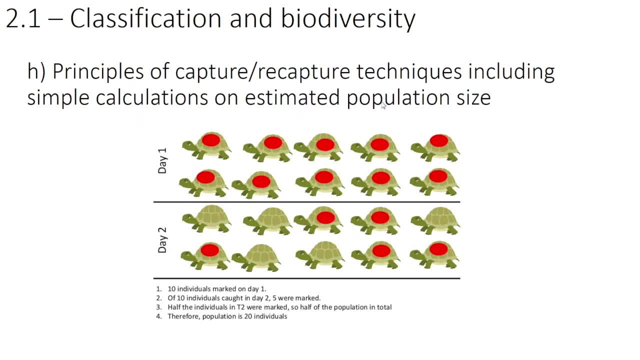 recapture techniques, including some simple calculations on estimated population size. This particular point is a higher level point, so if you're doing foundation paper for year 11- biology or science- you do not need to know this video. just move on to the next one, okay. but if you 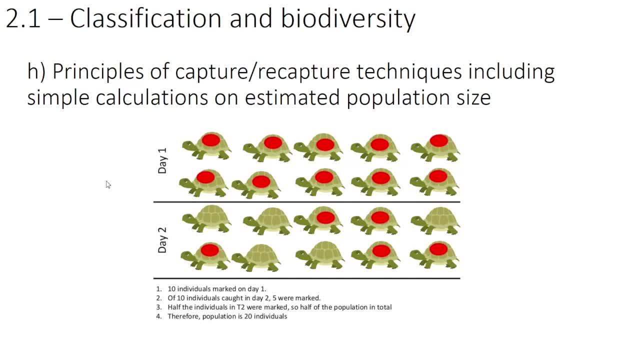 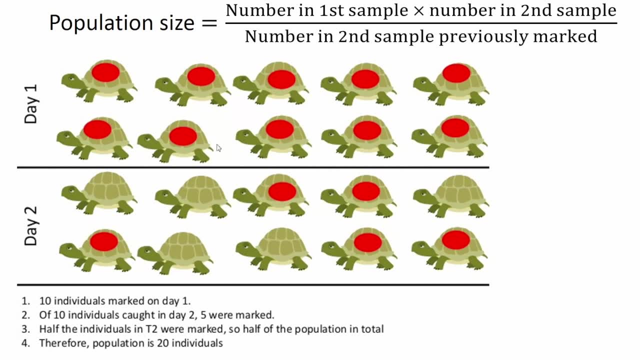 are doing higher, then you do need to know what this is all about. So we're actually going to be describing this picture in a lot more detail, so to make it a little bit bigger then. So we have here some turtles. okay, this technique is for animals- capturing and recapturing animals, and 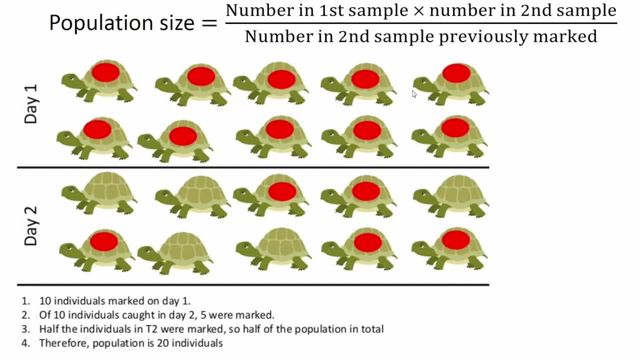 we can estimate a population size of animals by marking animals, releasing them back into the wild and then recapturing the same From the same area and then doing some maths to estimate population size. So we have one, two, three, four, five, six, seven, eight, nine, ten turtles that we are catching on day one. okay, On day two we have 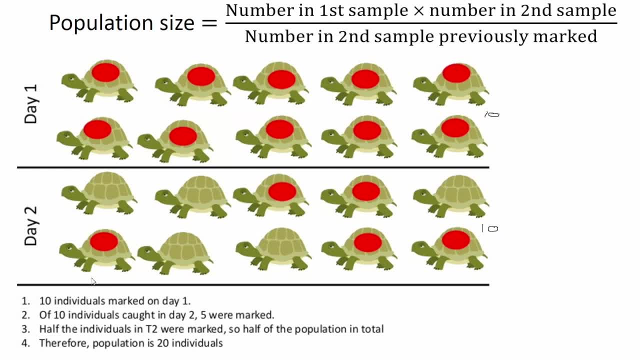 ten turtles again- and we'll talk about that in a minute- and it says down here: ten individuals are marked on day one. so we're going to investigate the population size of turtles. We have caught ten on our first day and we're going to mark them each with these red dots. 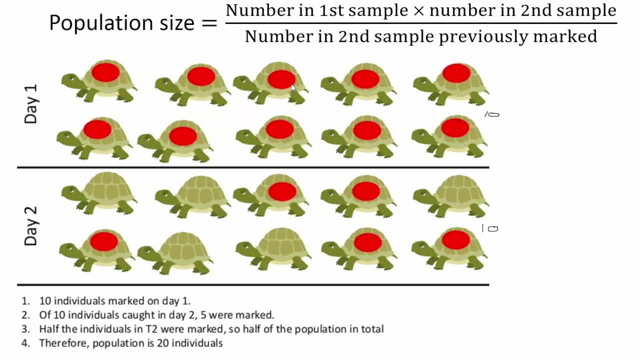 Okay, we're going to mark them. in reality they'd be a lot smaller than this. okay, then we're going to just release them back into the wild and wait. and then on day two, down here, we're going to take ten more turtles again. and then we've got ten turtles. some of them have the red dots and some of them. 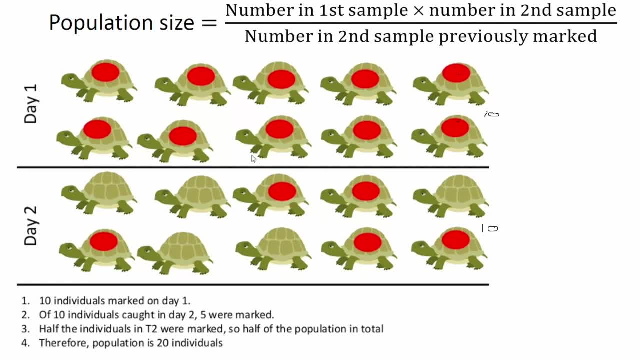 don't, which means that some of them we've caught once before in day one, and some of them we haven't. so of the ten that were caught in day two- it's saying this down here- five of them already marked: one, two, three, four, five. so five were marked and one, two, three, four, five were not marked. 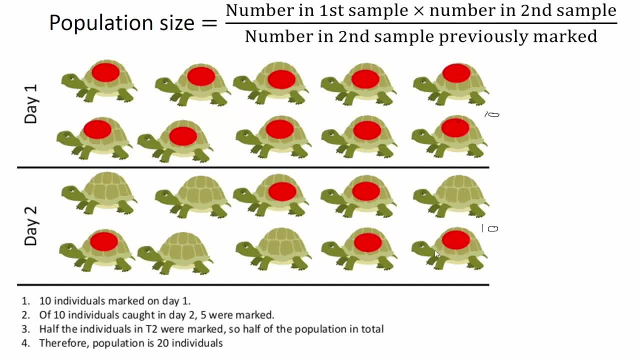 so half of the individuals here were marked and half weren't. so we had ten marked here and five marked here, and all we're going to do is input these numbers into the equation at the top of the page. I stress this: you do not need to memorize this. you don't need to know it. 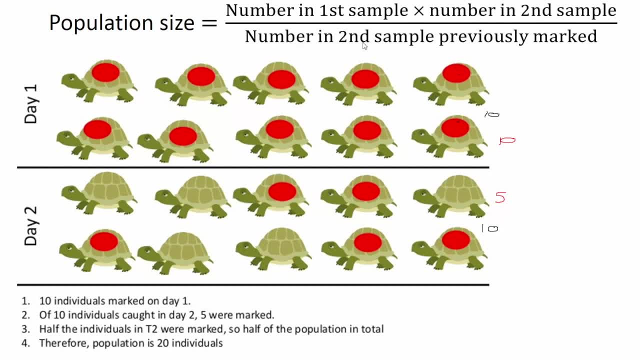 they will give it to you in the exam and if it's not in the question, it will be on the equation sheet at the front of the exam. refer to it, please, please do don't think you need to memorize these equations, you don't? so I'm going to put in the numbers. so population size of these. 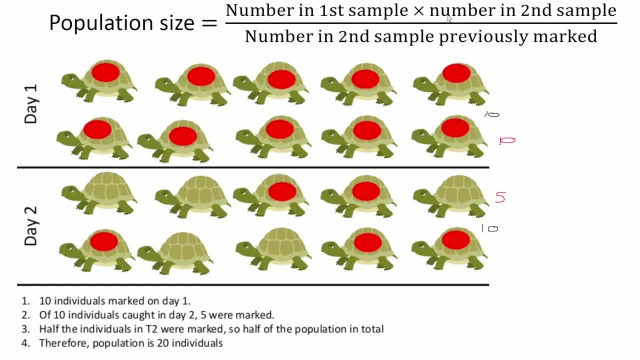 turtles equals the number in first sample times, the number in the second sample and that's just the total numbers, which for me was 10 and 10. so number in the first sample times the number in the second sample, 10 times 10 divided by what. so my last number is the number in the second sample that were previously marked. 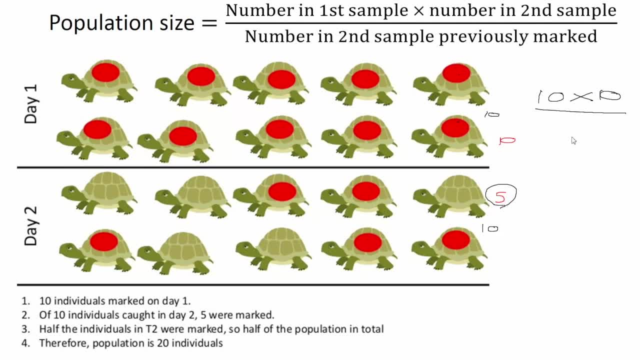 and this for me was this number here, this five, because five of them were previously marked and were found again. so we're going to divide by five. so me personally, because I'm not going to use a calculator, I'm just going to do this in my head- 10 times 10 is 100, 100 divided by 5. 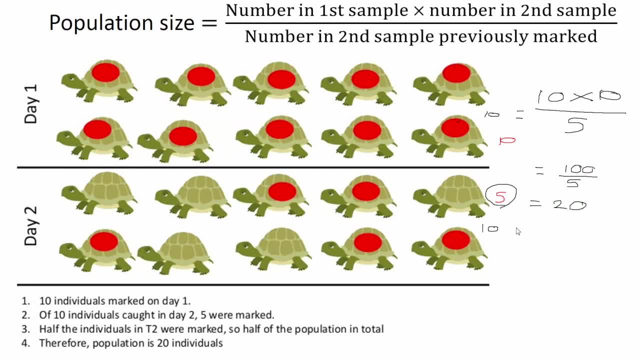 equals 20.. therefore, I am estimating there are 20 turtles in this environment. okay, now the numbers might get strange, but ultimately you're just doing the same thing again. so one time you take a sample, next time you take a sample, and then, when you compare how many you? 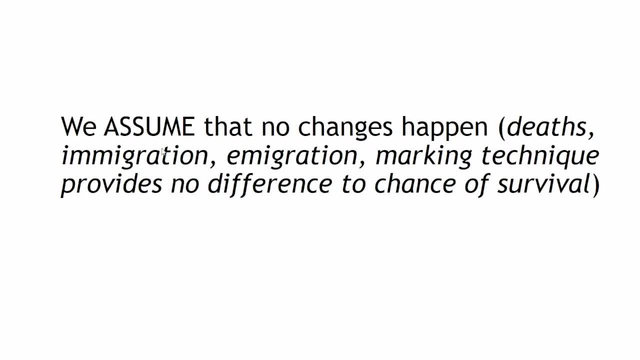 caught that were marked. that's all now. just like with quadrats, we are making assumptions during our investigation. we are assuming that no changes happen and this could be due to death. so some of the turtles could die overnight, and but we're assuming that none of that happens, so it does have. 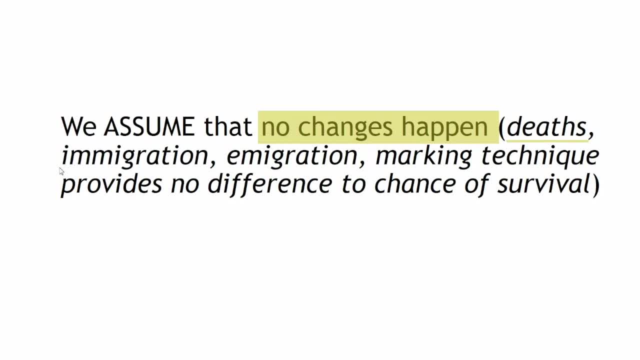 some flaws, you see, that's why we're doing this, so we're going to do that. now let's go back to the this method. we're also assuming that no immigration happens, which for animals is much more likely than for plants, and similarly with emigration out of the 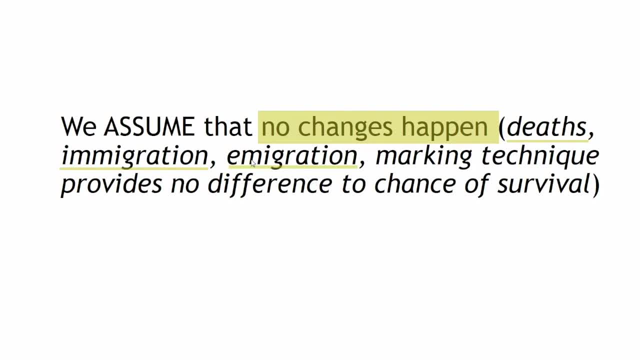 area. maybe us coming in scared them off and some of them left the area, so we're not sure if that could have had an effect on the results. and also we have to assume that the marking technique that we used provides no difference to the chance of survival, because you've got to imagine if we're put in a massive